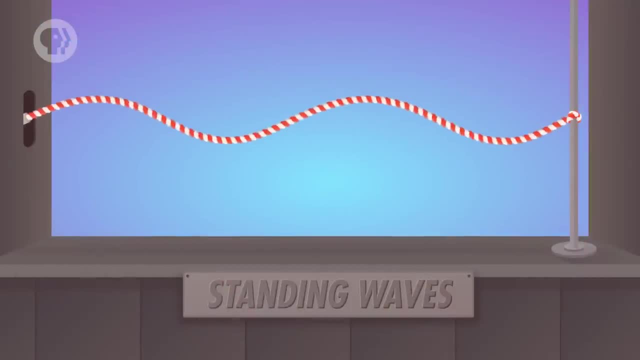 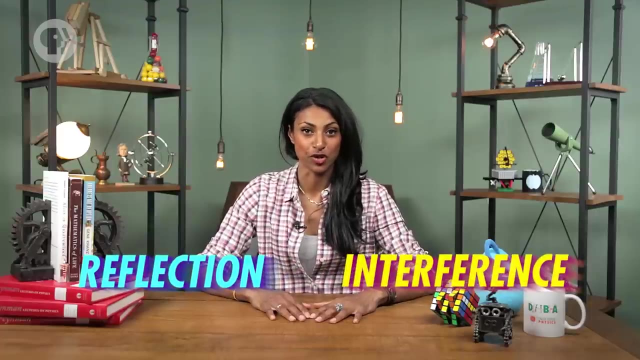 They're standing waves. A standing wave is a wave that looks like it isn't moving. Its amplitude may change, but it isn't travelling anywhere. Standing waves are the result of two other things waves do, both of which we've talked about before – reflection and interference. 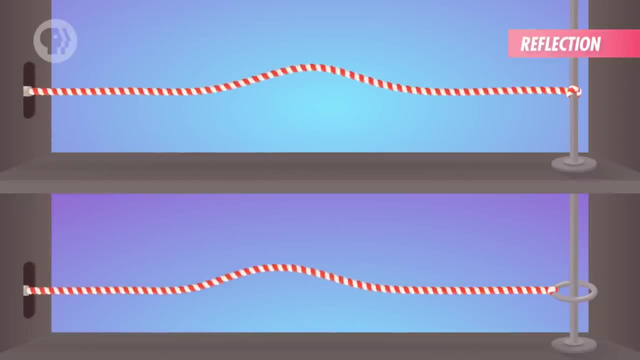 Reflection is what happens when a wave reaches the end of a path and then moves back along the same path. That's what happens when you send a pulse down a fixed rope: It reaches the end and then comes right back. When we send a continuous wave down a rope, that's when interference comes into play. 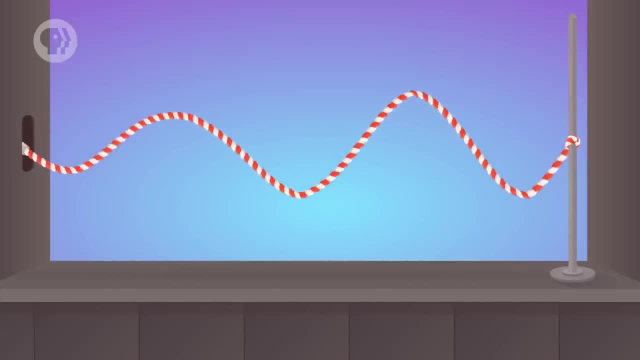 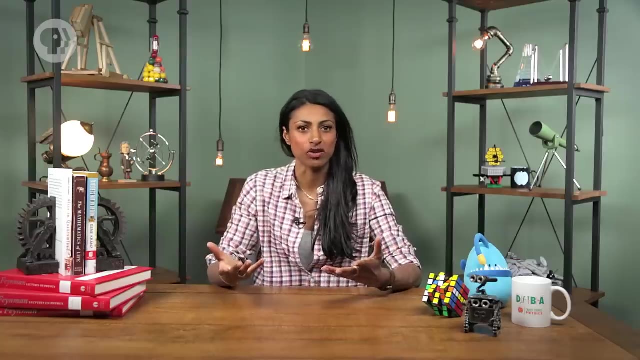 The wave reaches the end of the rope and is reflected, but there are more peaks on the way. As the peaks pass each other, they interfere with one another, changing their sizes. Usually you end up with crescent troughs that are different sizes and various distances apart. 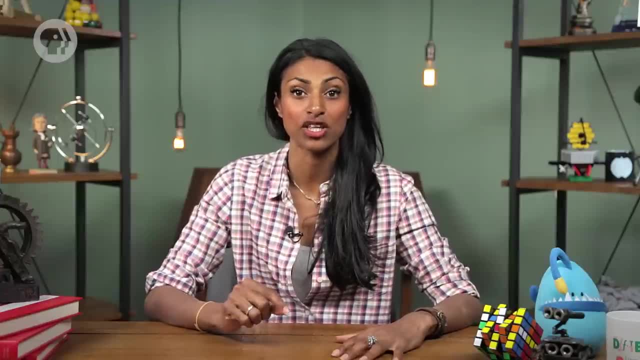 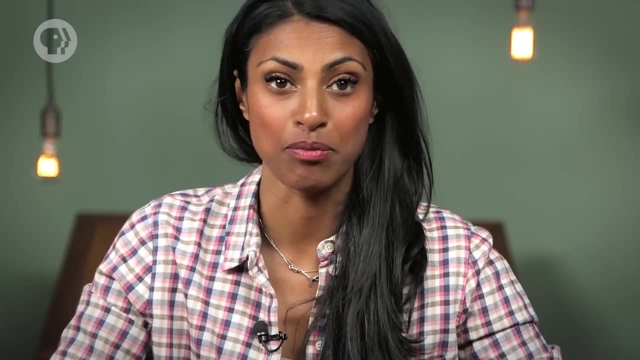 But at certain frequencies the reflective waves interfere in such a way that you end up with a wave that seems to stay perfectly still, with only its amplitude changing. That's a standing wave, And it can happen both in strings and in the air and pipes. 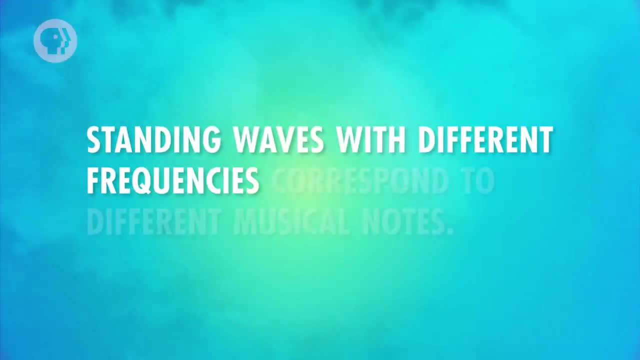 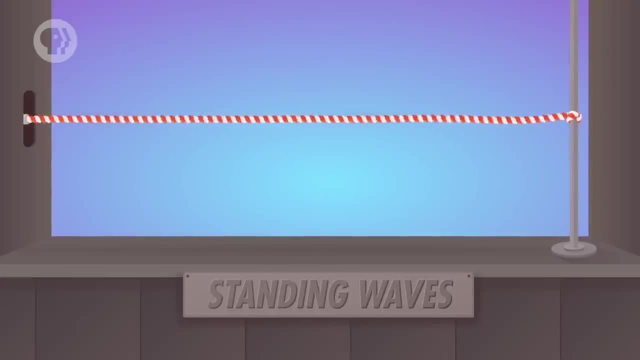 And that's what makes music. Standing waves with different frequencies correspond to different musical notes. Now, in order to understand how standing waves operate, you should get to know their anatomy. The points of a standing wave that don't oscillate are called nodes, and the points at maximum height of the peaks are antinodes. 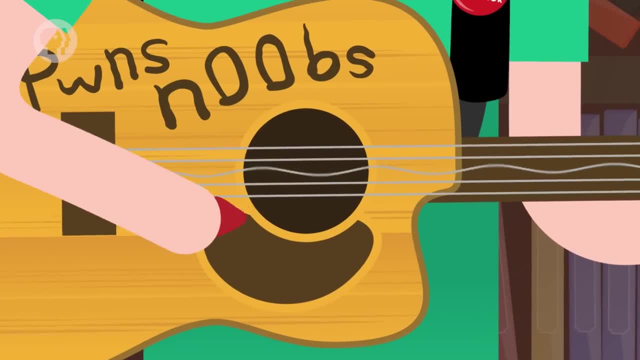 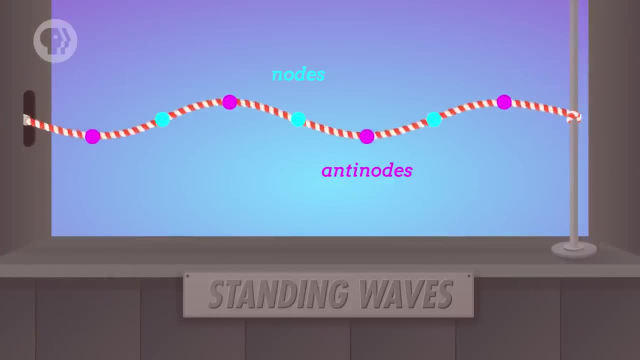 And here's something cool: If you look at a string on a stringed instrument as it's creating a sound wave, you can actually see where the nodes and antinodes are. The standing waves create peaks along the string, And between those peaks there are points that just stay still. 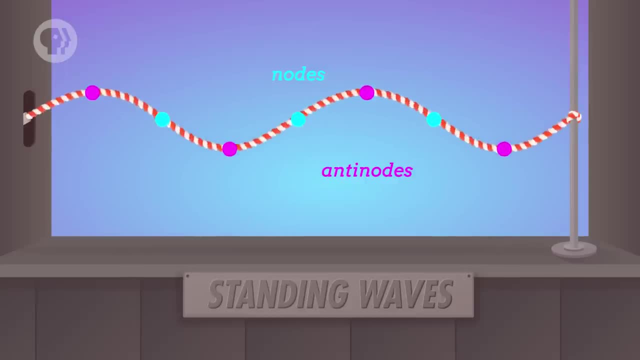 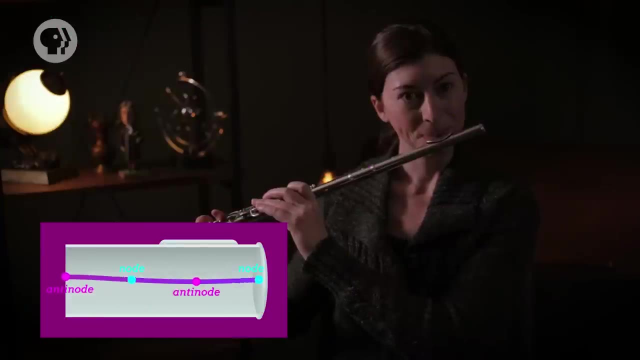 So the peaks are the antinodes and the points that don't oscillate are nodes, And if one or both of the string ends are fixed, then each fixed end is a node too, because it's stuck in place. Now in a pipe, the standing waves are made of air molecules moving back and forth. 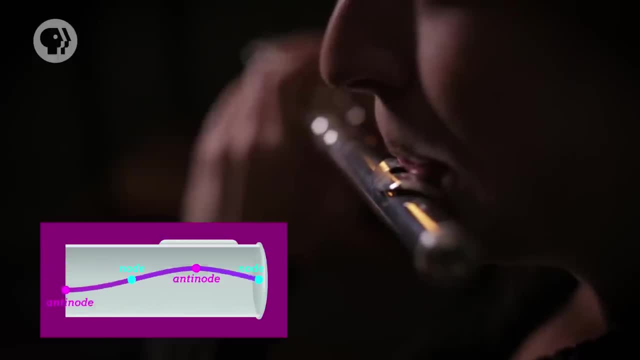 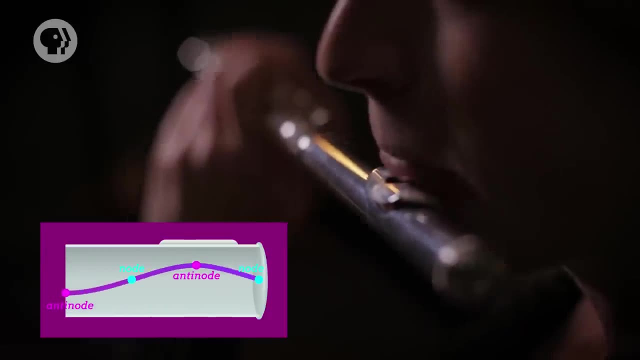 But the areas where molecules oscillate the most, including those near any open ends of the pipe, form the peaks and therefore the antinodes, And between those peaks, as well as any closed ends of the pipe, are areas where molecules don't move at all. 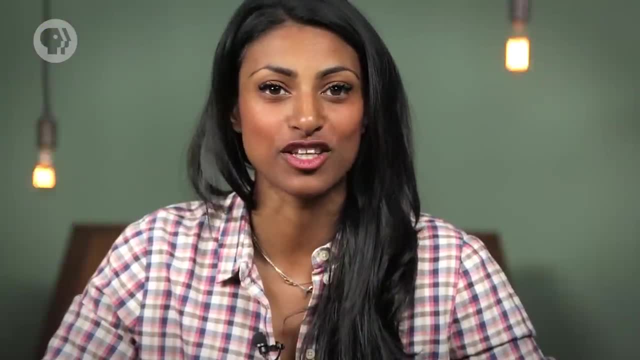 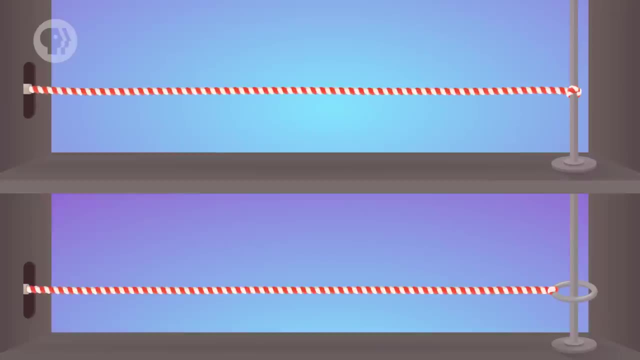 Those are the nodes. Generally, musicians make their music using the frequencies of these standing waves, But the nature of these waves depends a lot on what the ends of the string or pipe look like. Remember how a wave travelling down a rope gets reflected differently depending on whether the end of the rope is fixed or loose. 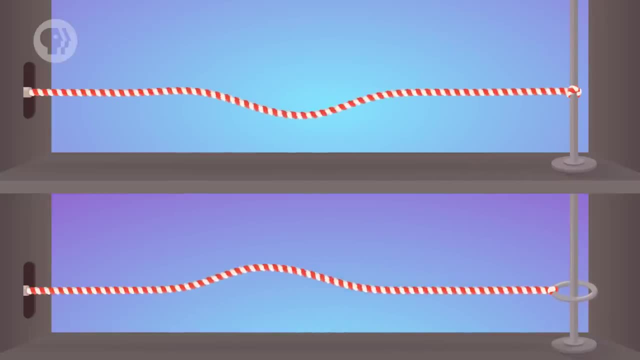 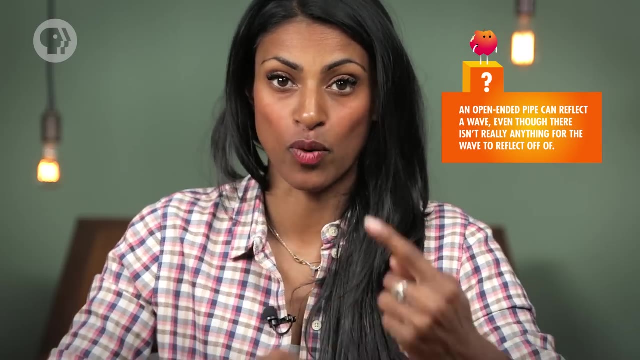 A fixed end will invert the wave, turning crests into troughs and vice versa, while a loose end will just reflect it without inverting it. The same thing holds true for air in a pipe: A closed end will invert the wave, while an open end won't. 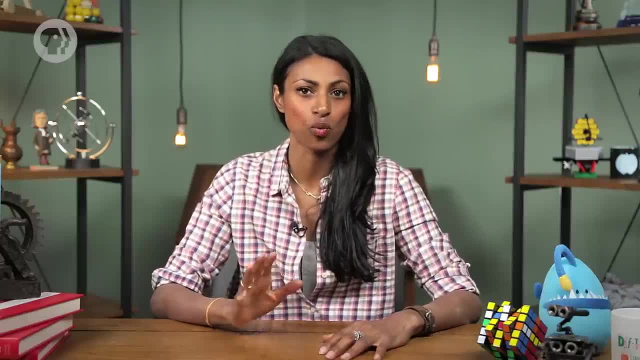 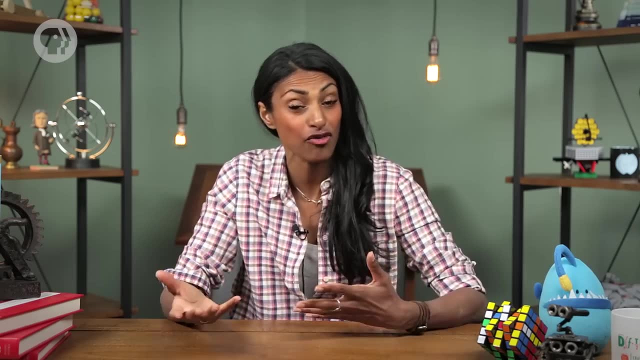 So the properties of a standing wave A standing wave will be a little different depending on whether it's made with a string with two ends fixed or a pipe with two ends open, or a string or a pipe with one end fixed and the other open. 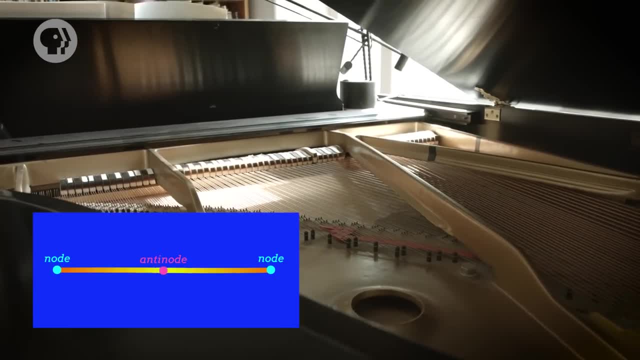 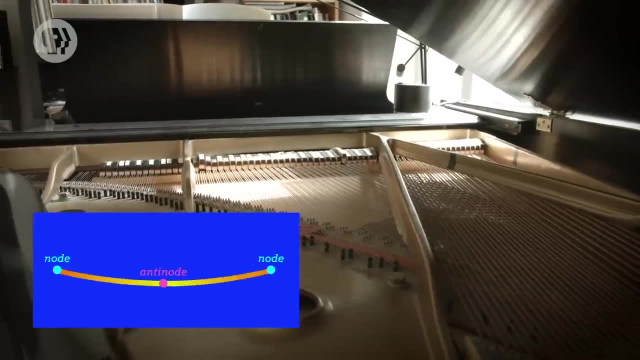 A string with two fixed ends, like in a piano, is probably the simplest way to understand standing waves, Because we know that, no matter what, the wave made by a fixed string will have at least two nodes, one at each end, And in its most basic form it would have just one antinode in the middle. 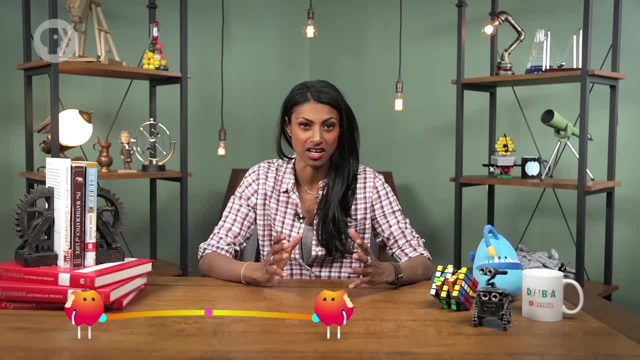 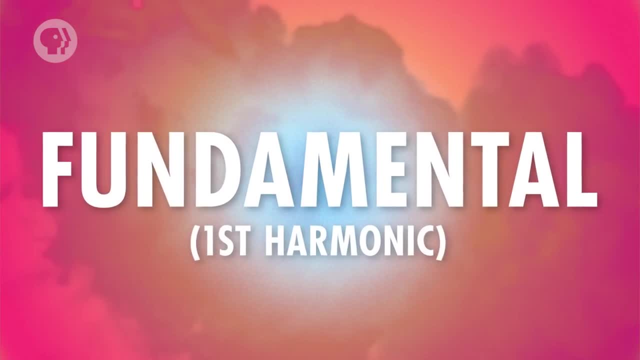 So the wave is basically a peak that moves from being a crest to a trough and vice versa, Like some kind of one-dimensional jump rope. This most basic kind of standing wave is known as the fundamental or the first harmonic. It's the simplest possible standing wave you can have, with the fewest nodes and antinodes. 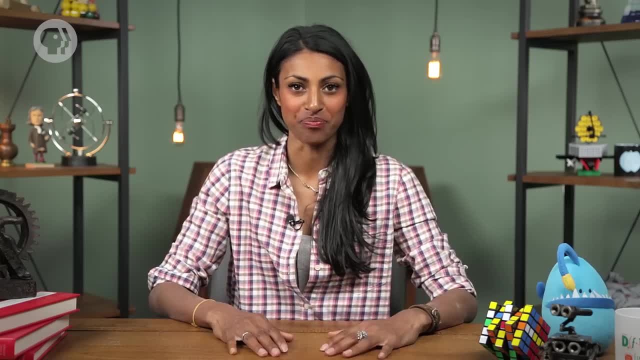 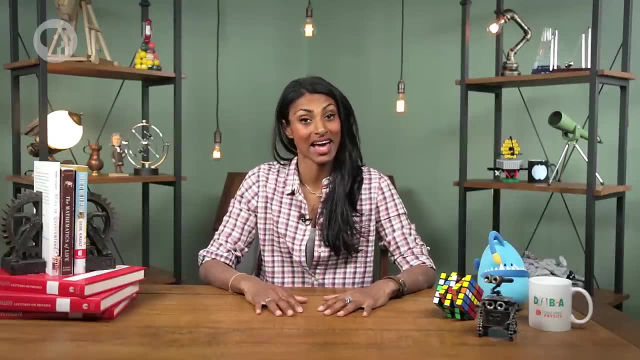 There are other, more complex standing waves that you can have too. These are known as overtones. Overtones build on the fundamental incrementally. Each overtone adds a node and an antinode, So each of these overtones is related to the fundamental wave and all of the overtones are related to each other. 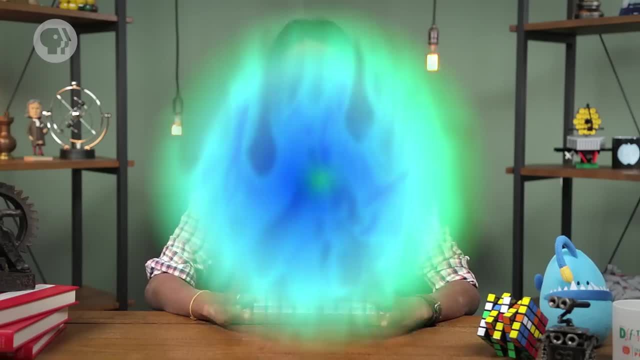 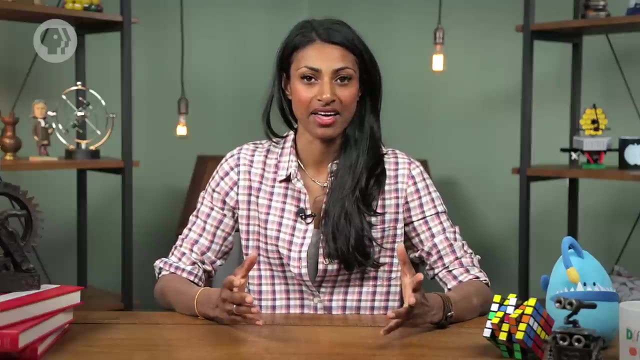 Together. the fundamental wave and the overtones make up what a node. The fundamental is the first harmonic and the overtones are higher-numbered harmonics. With each node and antinode pair that's added to the standing wave, the number of the harmonic goes up. 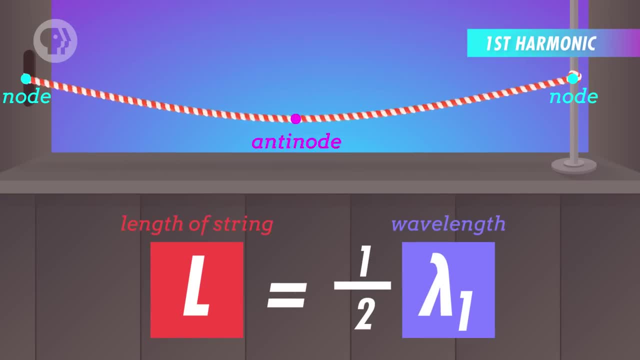 Second harmonic, third harmonic and so on. Now physicists sometimes express harmonics in terms of wavelength. For example, for a string with two fixed ends, you'll notice that the fundamental covers exactly half a wavelength. A full wavelength of the wave would span two peaks: a crest and a trough. 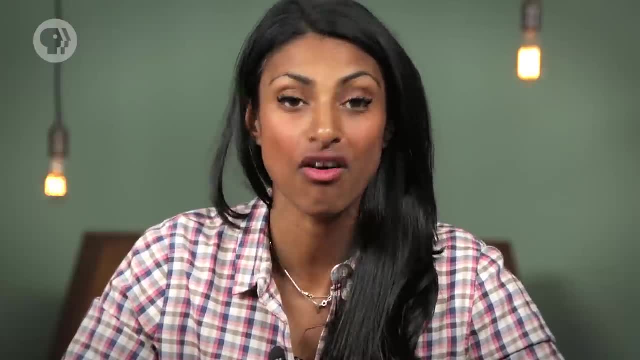 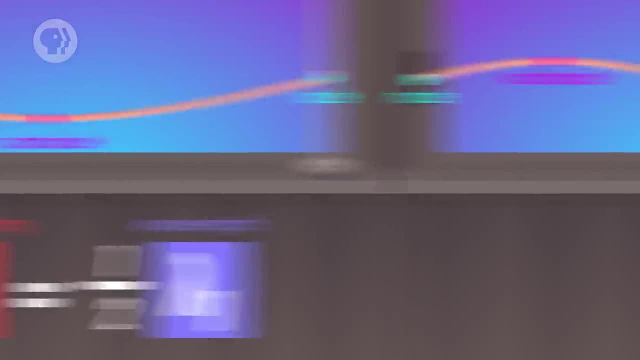 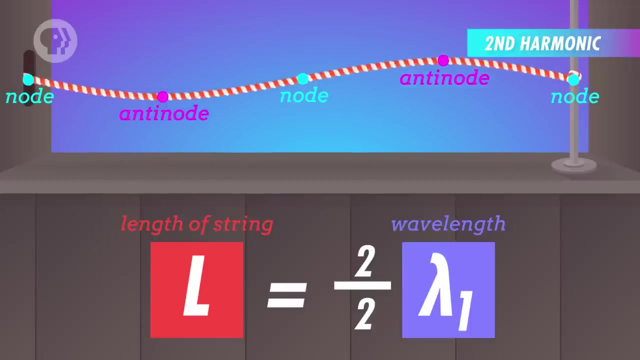 But the fundamental spans exactly one peak, which is half the wavelength. So for the fundamental of a string with two fixed ends the length of the string is equal to half a wavelength. The second simplest standing wave you can have on a string with two fixed ends has three nodes, one at each end and one in the middle, plus two antinodes between the nodes. 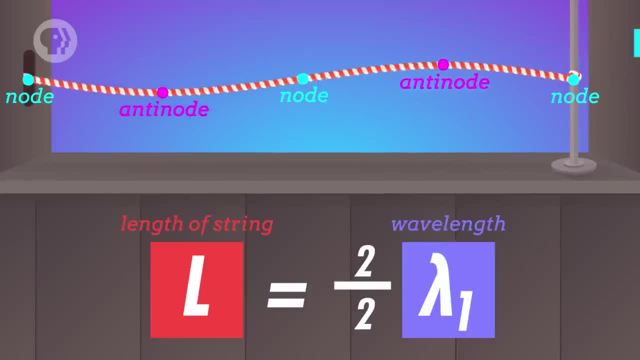 It's called the second harmonic and the string holds exactly one wavelength. You can probably guess what the third harmonic looks like: It has four nodes and three antinodes, and the string holds 1.5, or 3 over 2, wavelengths. 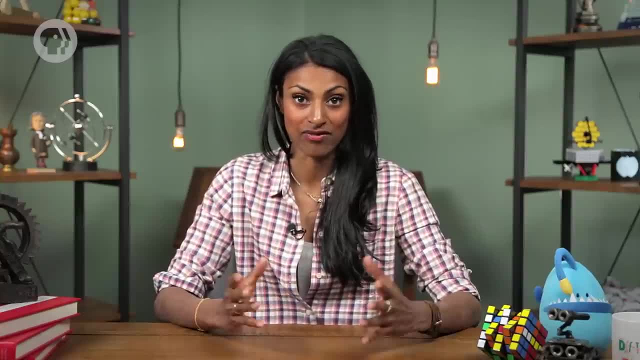 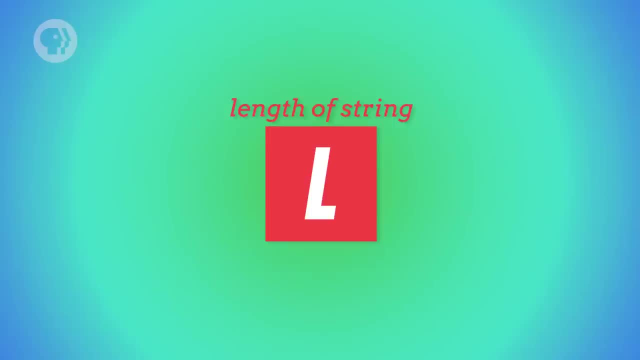 You may have started to notice a pattern For a standing wave on a given length of string. the number of wavelengths that fit on the string is equal to the number of the harmonic divided by 2.. So now we have an equation that relates the wavelength of a standing wave to the number of the harmonic and the length of the string. 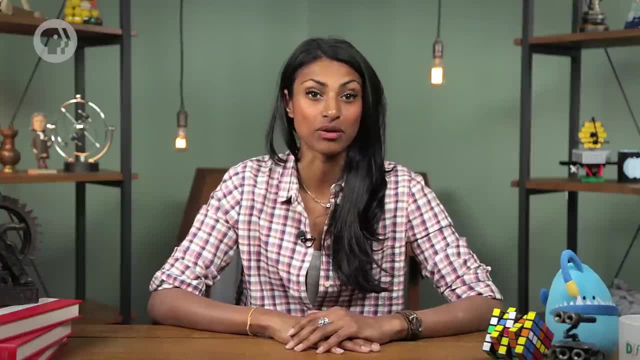 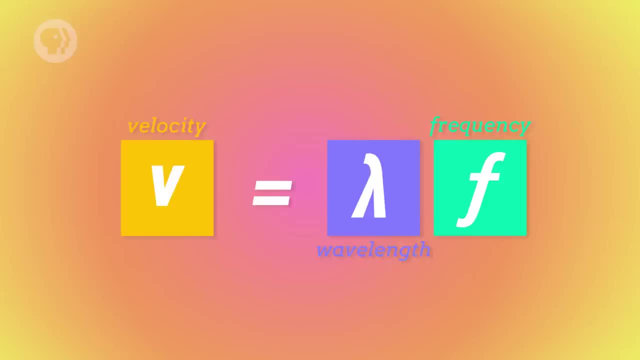 Once you get a handle on the wavelength, you can figure out the aspect of the wave that musicians care about most – the frequency. We've already established that a wave's wavelength times its frequency is equal to its velocity, which will be the same for each harmonic, because a wave's velocity only depends on the medium it's traveling through. 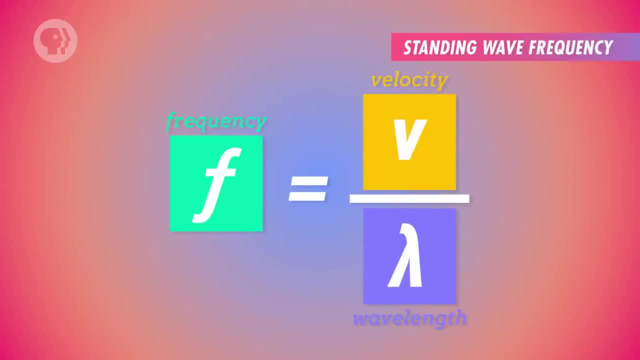 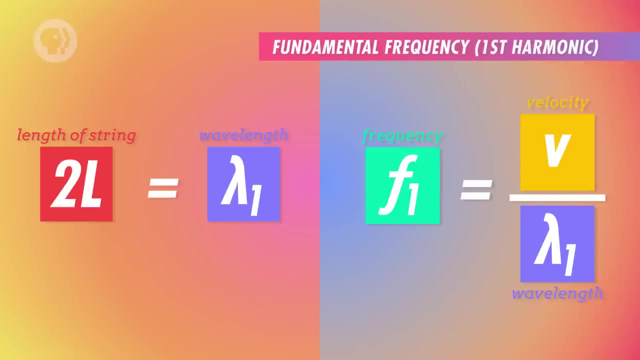 So a standing wave's frequency will be equal to its velocity divided by its wavelength. For the fundamental with two fixed ends, we already know that the wavelength is twice the string's length. So the frequency of that fundamental standing wave, known as the fundamental frequency, is equal to the velocity divided by twice the length of the string. 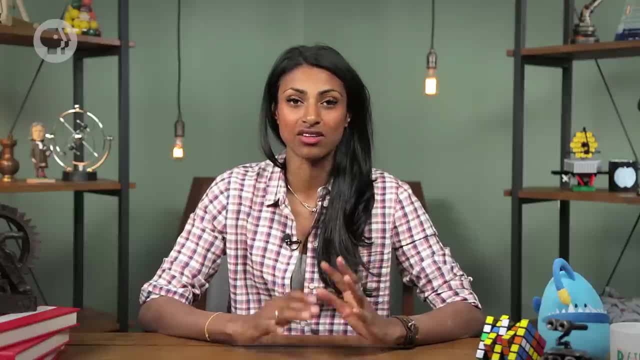 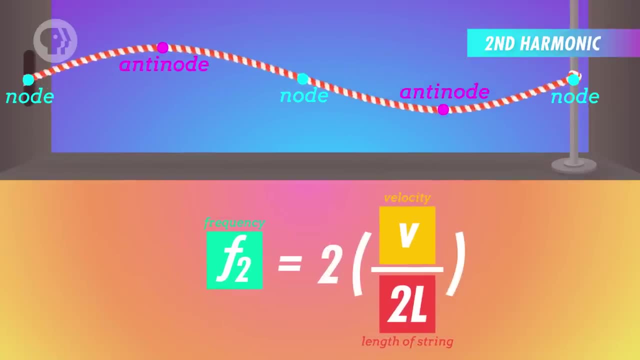 We write it as f, with a subscript of 1.. Now, what about the frequency of the second harmonic, the standing wave? with three nodes and two antinodes, It will be equal to the velocity divided by the length of the string, which is twice the fundamental frequency. 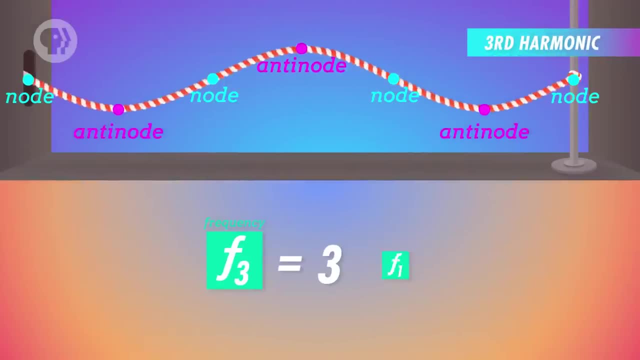 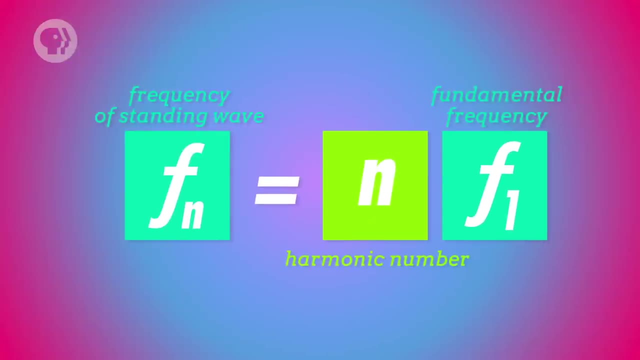 The frequency of the third harmonic, with its four nodes and three antinodes, will be equal to three times the fundamental frequency. So we're starting to see another pattern here. The frequency of a standing wave with two fixed ends will just be equal to the number of the harmonic times, the fundamental frequency. 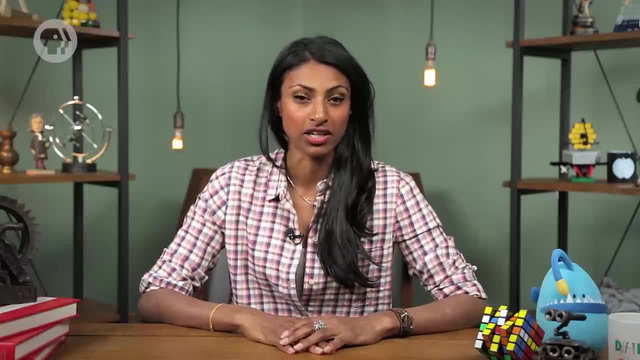 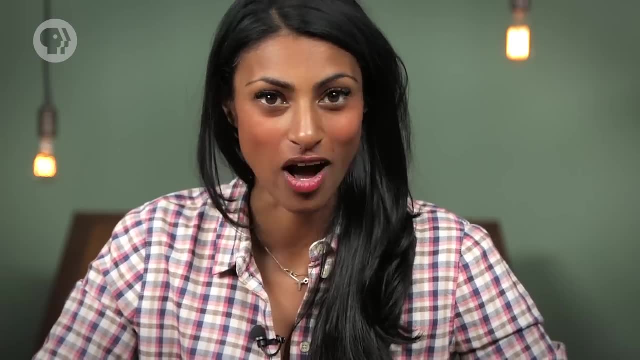 In fact that's one way to define harmonics. The number of a harmonic is equal to the number you multiply by the fundamental frequency to get the harmonic's frequency. This math is what makes musical instruments work. When you press down on a key on a piano, you make a hammer strike a string, creating standing waves in that string. 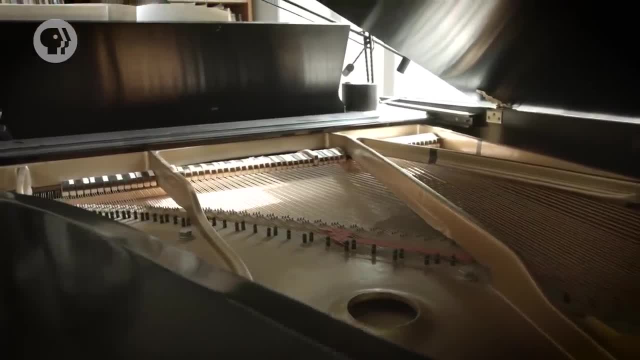 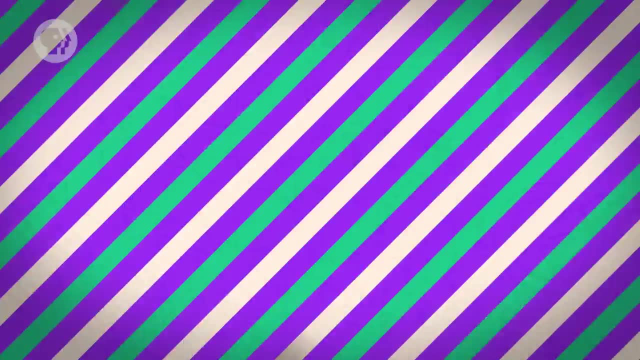 Every string in a piano is tuned so that its fundamental frequency, which depends on its length, mass and tension, corresponds to a given note. The middle C, for example, is 261.6 Hz. Guitars are also tuned so that the fundamental frequencies of their strings correspond to set notes. 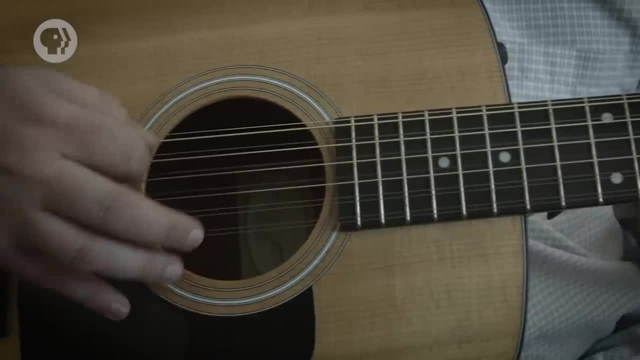 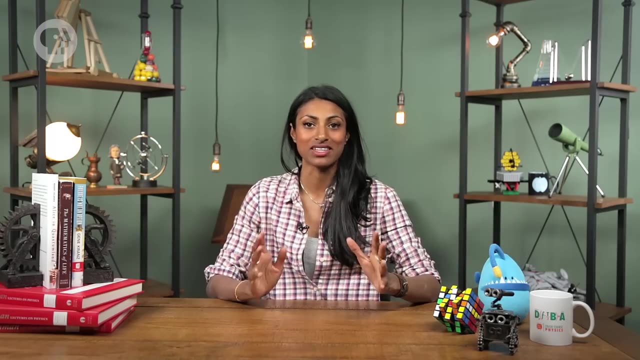 And when you press down on the strings in certain places you change the length of the active part of the string so that its fundamental frequency corresponds to a different note. So for a standing wave with two fixed ends we can relate wavelength, frequency, velocity, the length of the string and the number of the harmonic. 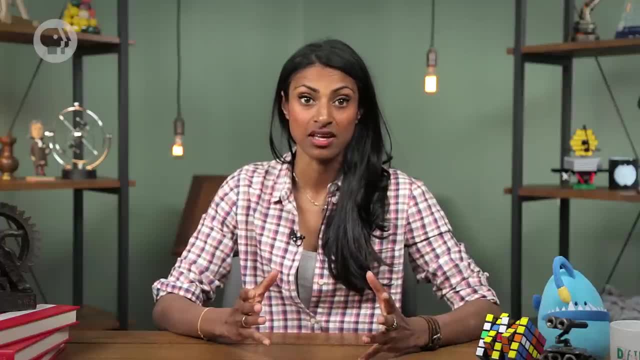 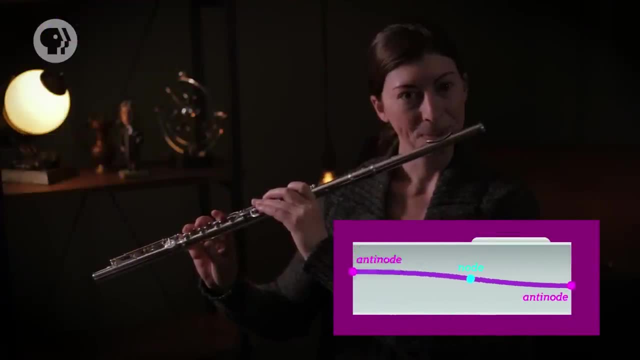 And we can do the exact same thing for a standing wave with two loose ends in an open pipe, for example, like in a flute. A standing wave in a pipe with two open ends is kind of the opposite of the wave with two fixed ends. 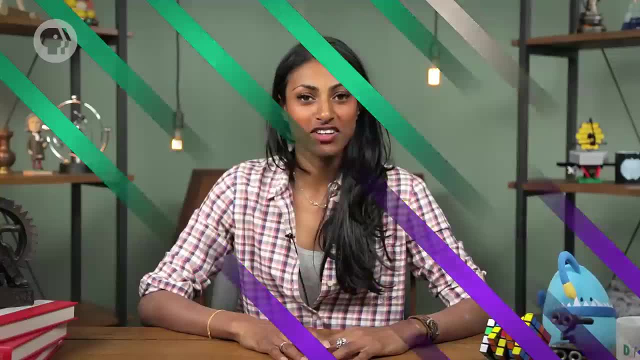 Instead of having a node at each end, it has an antinode at each end. So the fundamental standing wave for a pipe with two open ends will have two antinodes and one node in the middle of the wave. Then the second half of the wave will have two open ends. 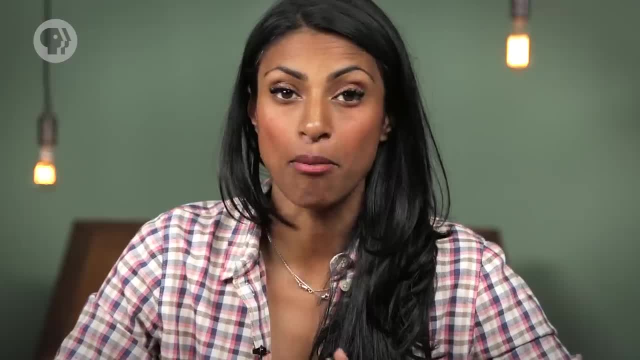 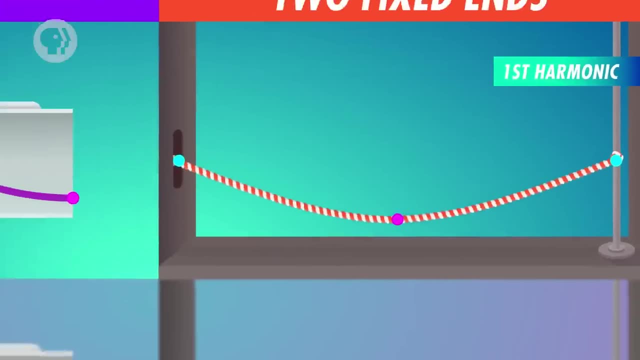 Then the second harmonic will have three antinodes and two nodes and so on, But each harmonic still covers the same number of wavelengths. Remember how the fundamental wave for a string with two fixed ends covered half a wavelength. The fundamental wave for a pipe with two open ends also covers half a wavelength. 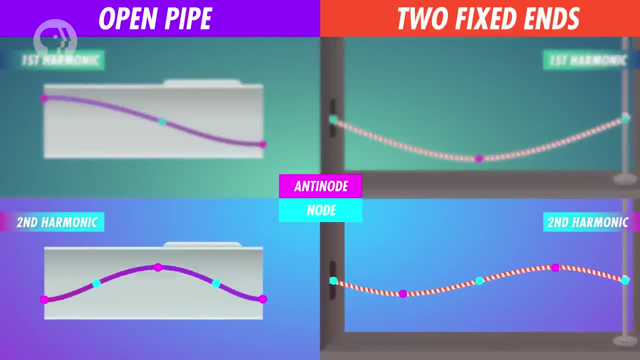 That half is just in a different section of the wave And just like a string with two fixed ends. the second harmonic for a pipe with two open ends also covers a full wavelength. It's just that in the case of a pipe, the wave starts and ends with a peak instead of a node. 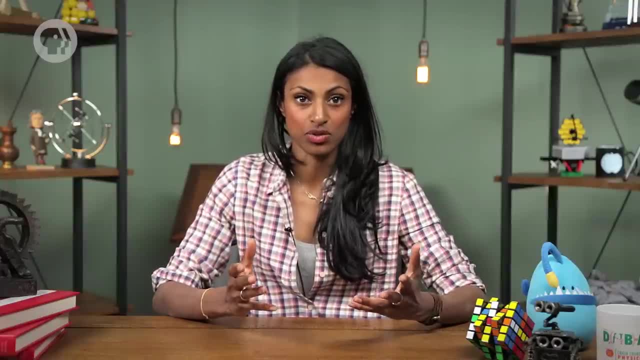 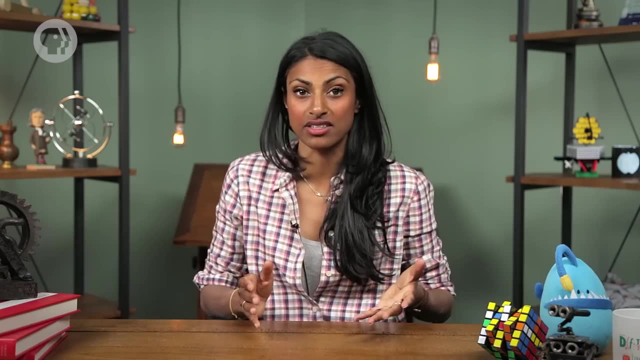 So the equations for wavelength and frequency are the same, And frequency for a standing wave with two open ends will be the same as they were for a standing wave with two fixed ends. So we've covered guitars and pianos and flutes. But a pipe with one closed end and one open end works a little differently. 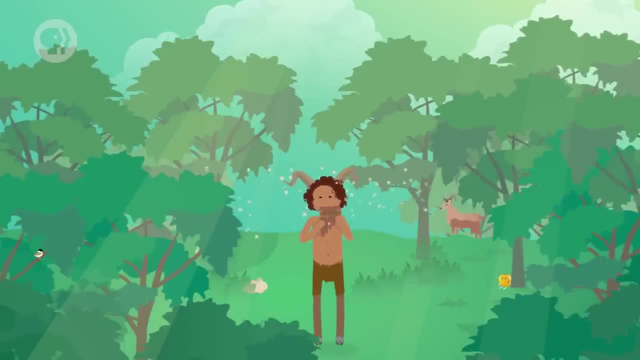 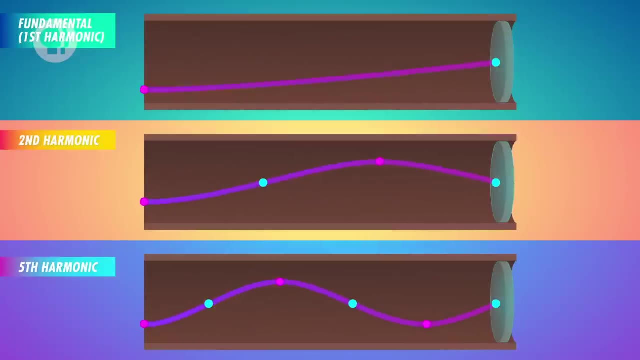 These kinds of pipes are used in instruments like pan flutes, where you blow across the top of a closed pipe to make music. Here standing waves need a separate set of equations for a couple of reasons. First, the closed end of the pipe will be a node because the air molecules aren't oscillating there. 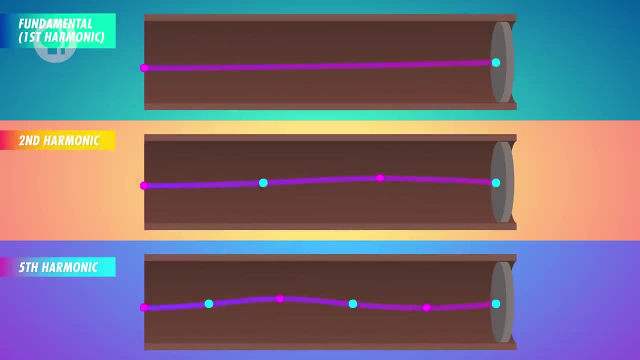 And the open end will be an antinode because that's where there's a peak in the oscillations, Which means that the simplest way to know if an open end is an antinode is when the air molecules aren't oscillating there And the open end will be an antinode because that's where there's a peak in the oscillations. 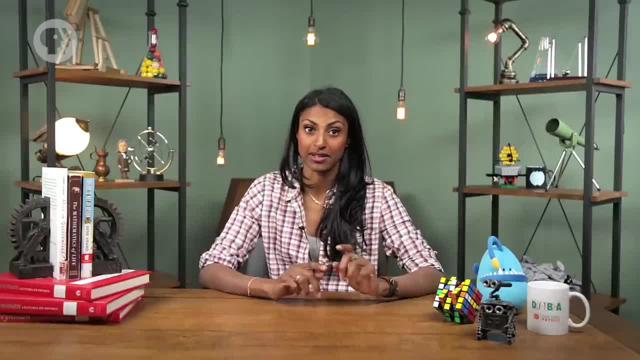 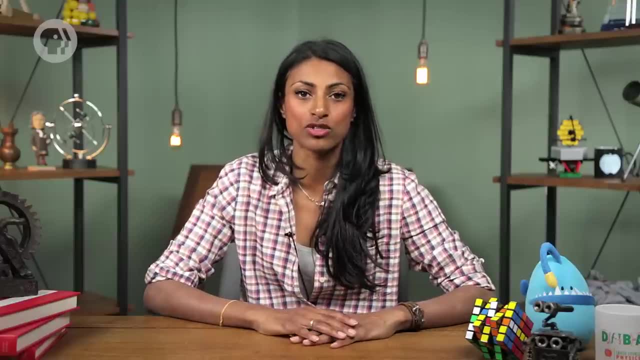 And the simplest way you can make in this pipe will stretch from one node to one peak. But that's only a span of a quarter of a wavelength in the pipe. Before, with both a string fixed at both ends and an open pipe, the fundamentals spanned half a wavelength. 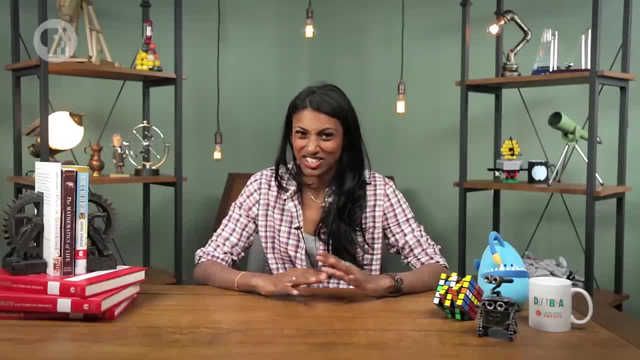 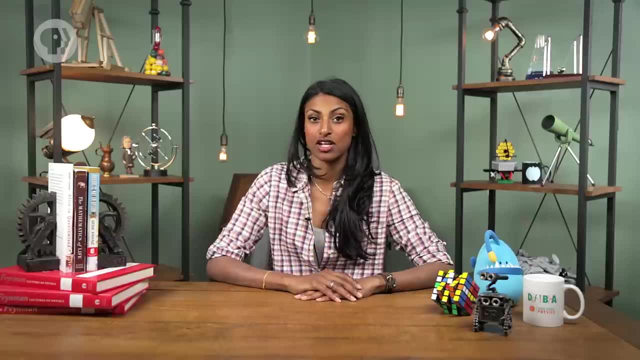 The fact that a pan flute pipe only covers a quarter of a wavelength changes things Because, remember, the frequency of each harmonic is equal to the number of the harmonic times, the fundamental frequency. But for a pipe that's closed on one end, you can't double the fundamental frequency, or quadruple it, or multiply it by any even number.